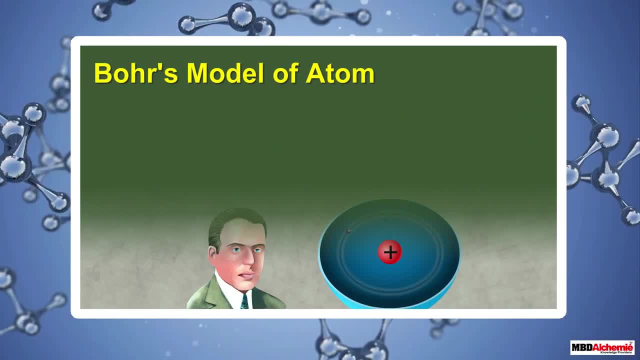 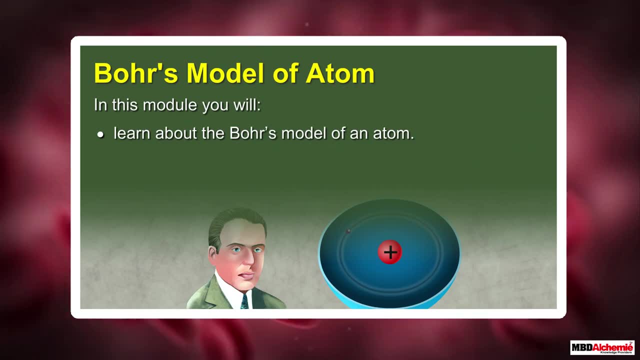 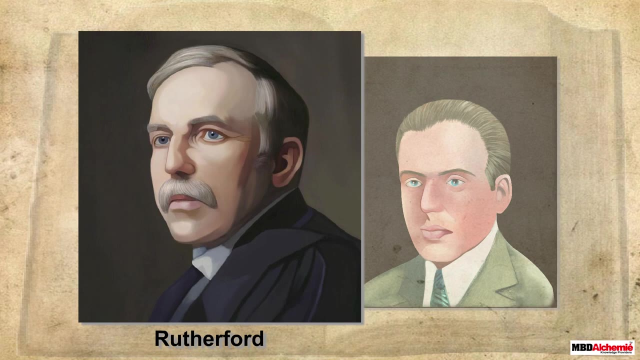 Bohr's model of an atom. In this module, you will learn about the Bohr's model of an atom. Prior to Bohr, there were a number of scientists who were working on the structure of atom. Rutherford was one of them, and his model was. 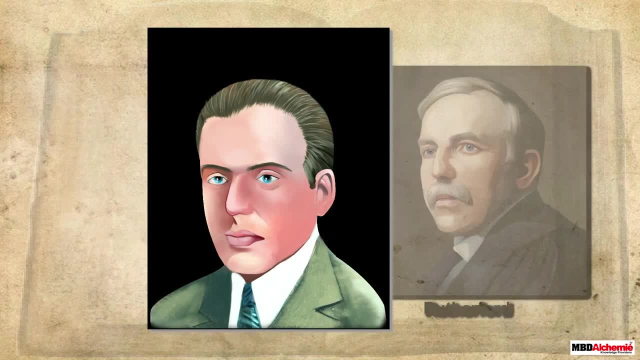 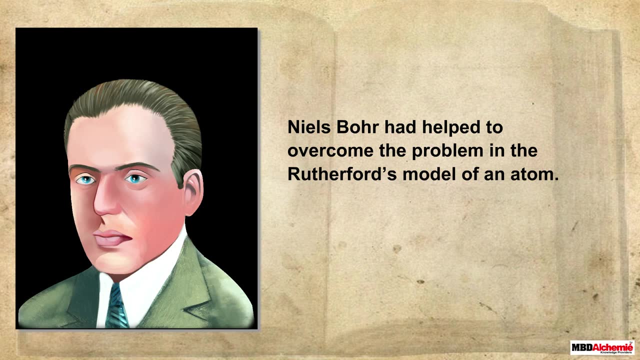 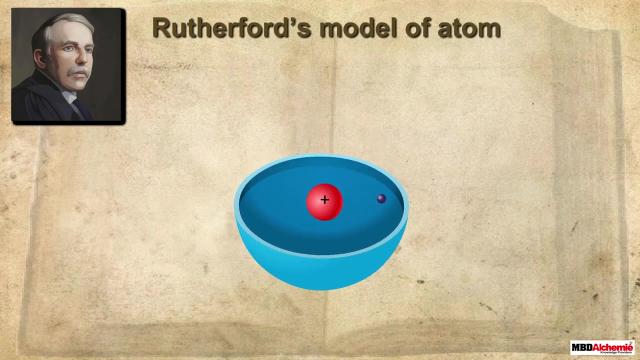 the closest model to the Bohr model of atom. In fact, Niels Bohr had helped to overcome the problem in the Rutherford's model of an atom. The Rutherford's model of an atom had a major drawback: that it could not explain the stability. 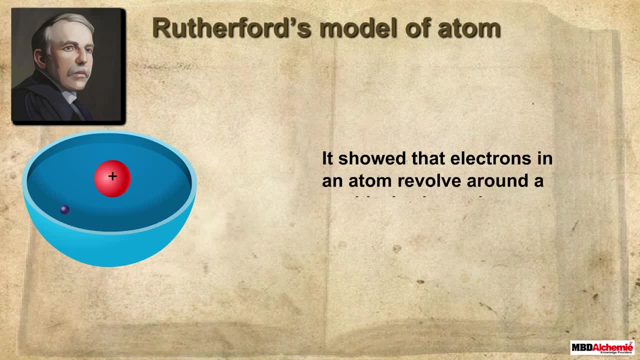 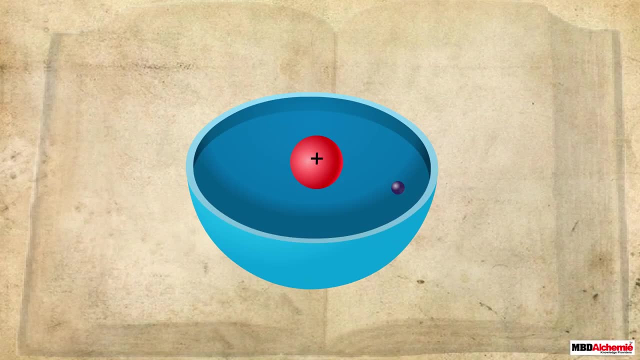 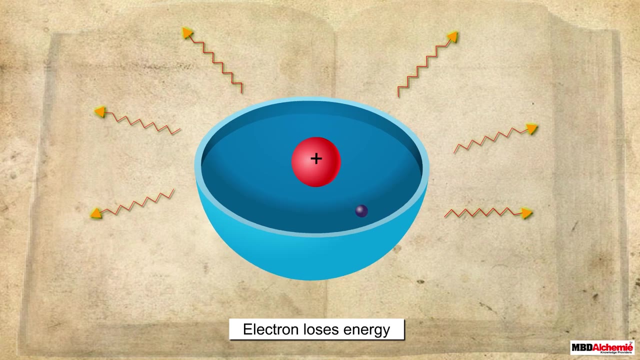 It showed that electrons in an atom revolve around a positively charged center called nucleus. However, later on it was found that any particle in a circular motion would undergo acceleration and thus would lose energy. So the electron would take a spiral path and would finally fall into the nucleus and the 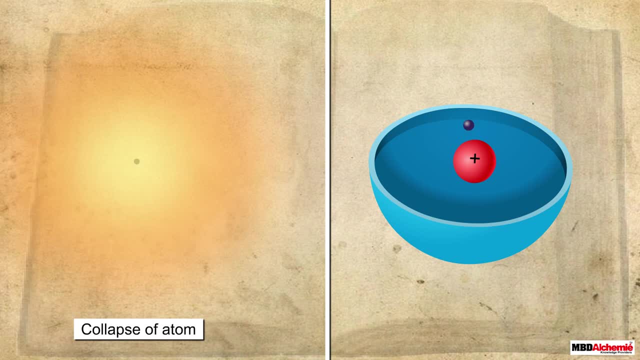 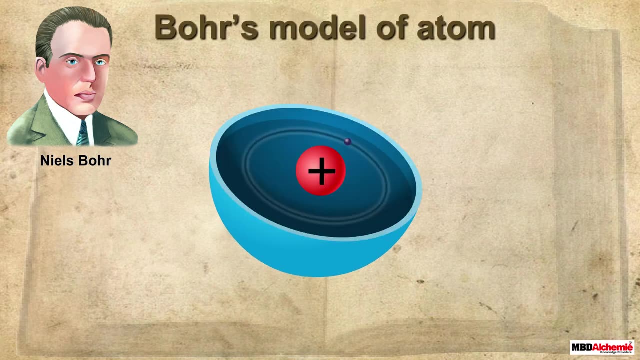 atom would collapse, But this does not take place in reality. Bohr said that electrons do revolve around the nucleus, but their energy remains fixed. He explained that the energy of electrons remains fixed because they are restricted to some fixed orbits. Each of these orbits is at a fixed distance. 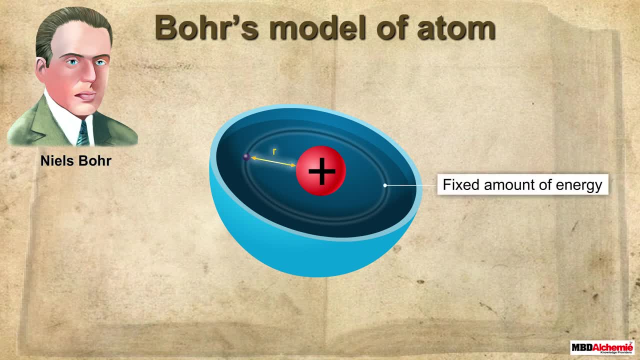 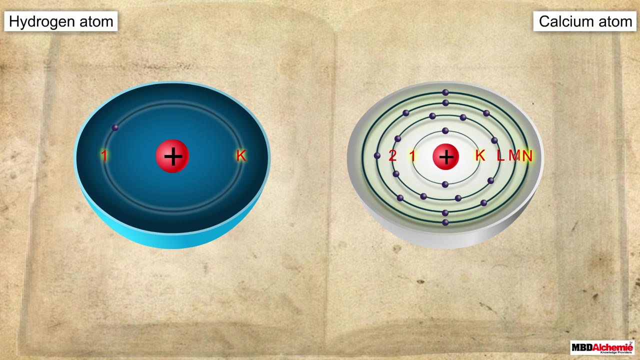 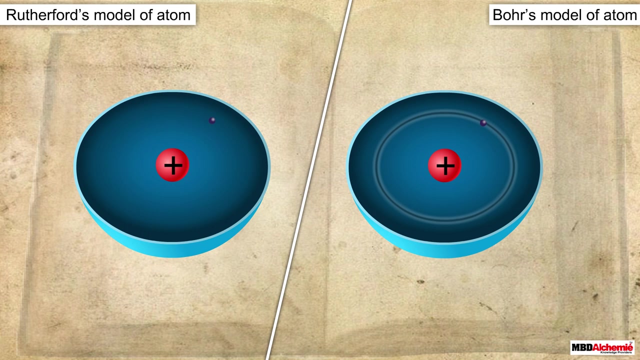 from the nucleus and is associated with a fixed amount of energy. These orbits with fixed energy are known as discrete orbits or energy levels. These energy levels are represented by the letters KLMN or the numbers 1234, starting from the center. So the final model of Niels Bohr was similar to the Rutherford's model of an atom which 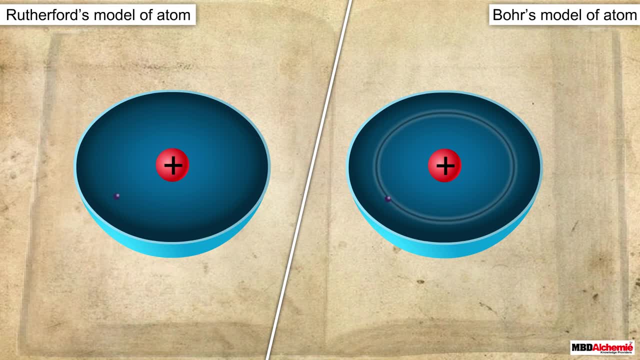 states that an atom consists of a positive and negative energy. So the final model of Niels Bohr was similar to the Rutherford's model of an atom, which states that an atom consists of a positive, negative energy, positively charged center, around which the electrons revolve. The only difference was: 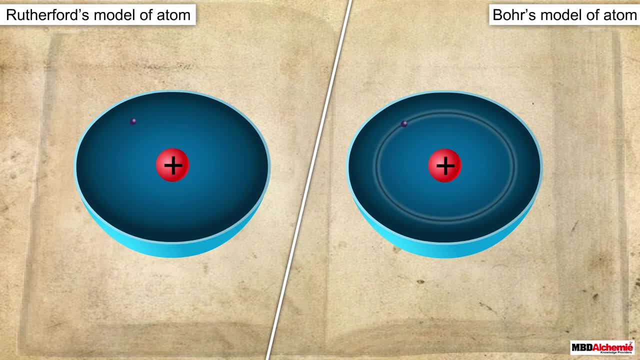 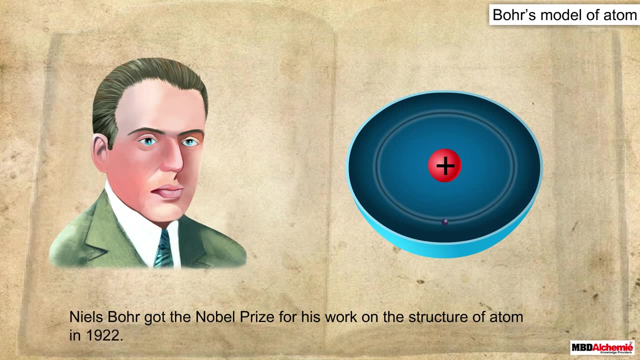 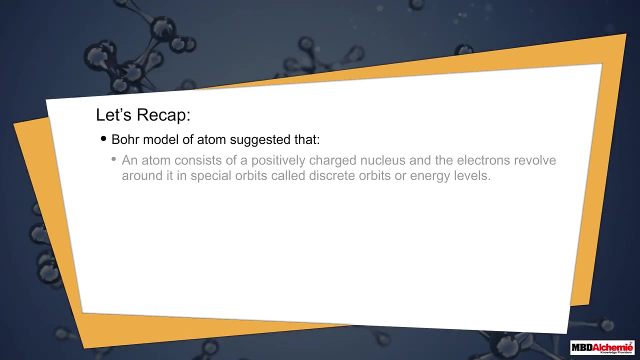 that in the Bohr model, electrons revolve around a nucleus in fixed orbits with fixed energy. For his work on structure of atom he got a Nobel Prize in 1922.. Let's recap: Bohr model of atom suggested that an atom consists of a positively charged nucleus.